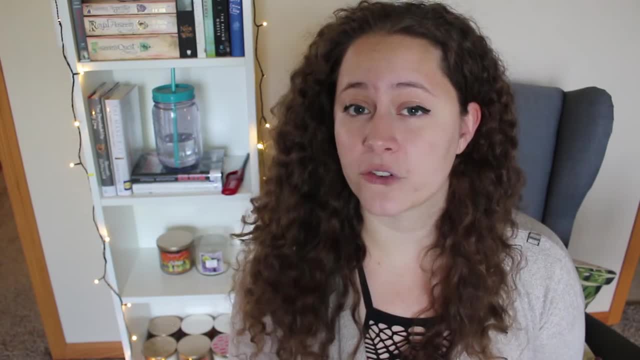 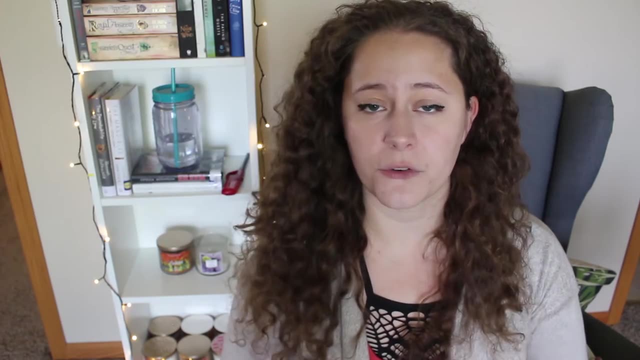 this effect, The movement of a fault can create what is known as a fault scarp, which we have talked about before, which in and of itself is not particularly dangerous, unless you have built your house directly on top of a fault. Now that primary effect of ground shaking actually causes most of these others. 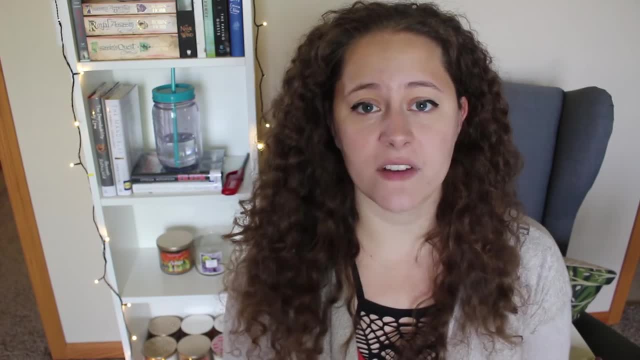 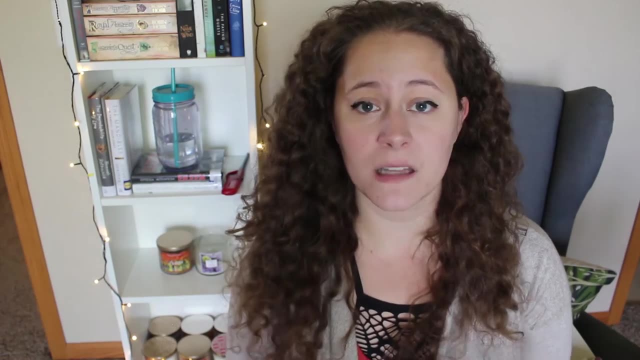 which is why it's known as a secondary effect. Landslides, avalanches and rock slumps can also be triggered by ground shaking, especially if you have a very unstable section of rock. A lot of the time, a rock slide or rock slump is more. destructive than the actual seismic waves. In 1948, an earthquake in the United States caused an earthquake in the United States that occurred high in the Andes Mountains south of Quito, and while that may not have been very destructive due to the lack of structures that are up there, it 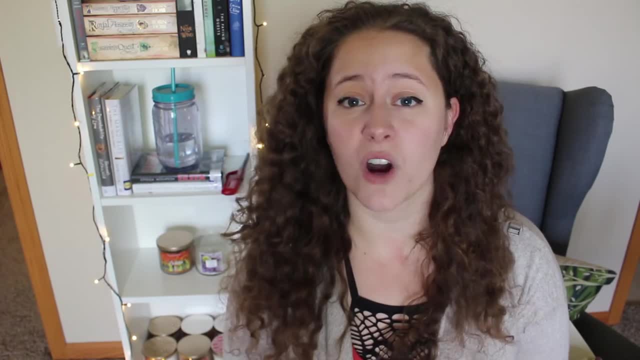 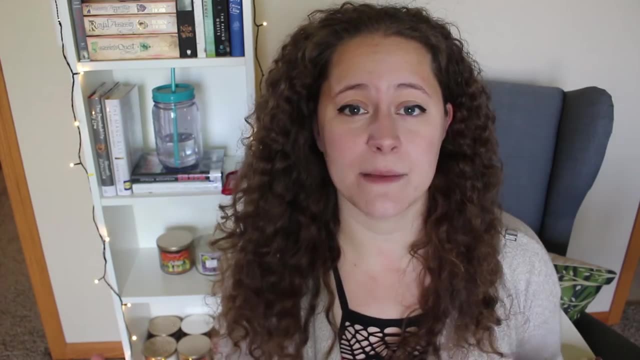 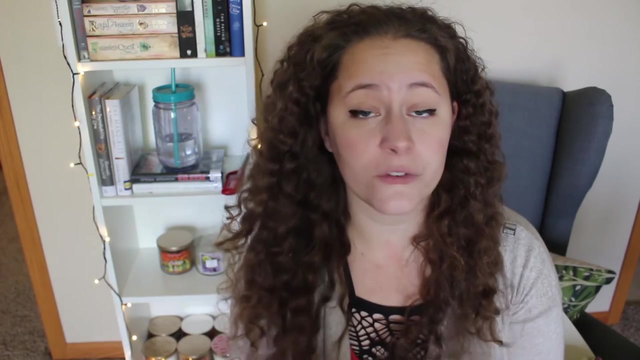 caused a landslide which killed 6,000 people and over a hundred thousand people lost their homes. Another one of these secondary effects is liquefaction. Liquefaction, kind of like the name suggests, is when something turns more liquidy. The shaking of an earthquake will stir up groundwater and soil and turn it more into a quicksand, like consistency. This obviously would also cause the foundations to sink and the building to collapse. Like most things, this depends a lot on the local geology. so if you have very sandy soil or if you have groundwater that is closer to the surface, you are 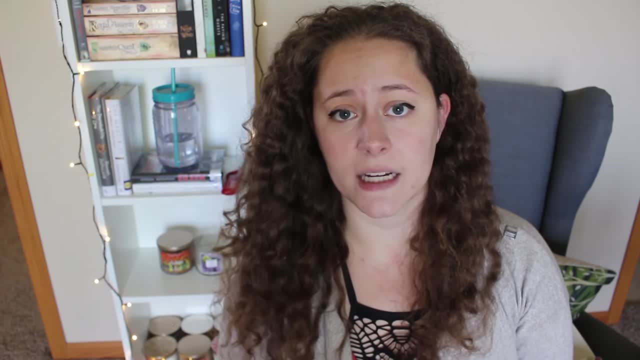 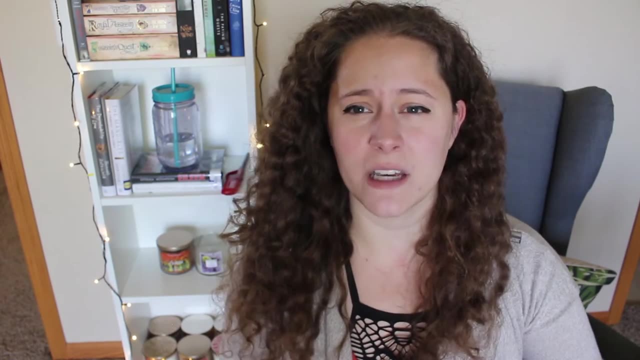 more likely to see this occur. Flooding is another secondary effect that we see a lot with earthquakes and can be a little bit confusing, because an earthquake by itself does not really involve a lot of water, Unless, of course, you're dealing with tsunamis, but then even news and media and weather. outlets tend to call them tsunamis and not link them back to the original earthquake. Technically, a tsunami is just a really big wave, but flooding can be caused by quite a few other things as well as the huge tsunami wave It can be. 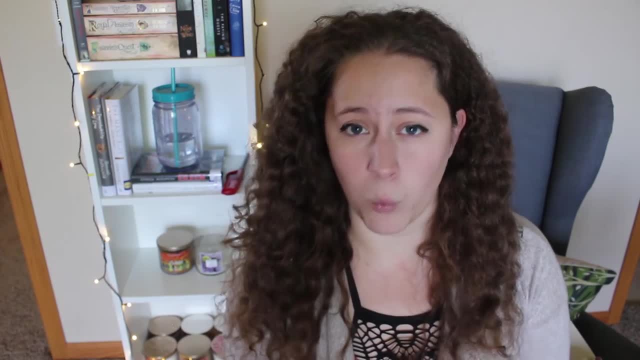 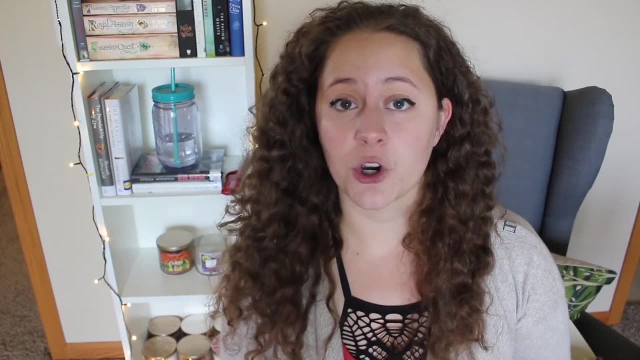 caused by a local river or lake. but even if you're not near water, broken water lines can also be a major cause of flooding. Now, if you do live next to a river or a lake, flooding can occur due to a phenomenon called a seiche. A seiche- 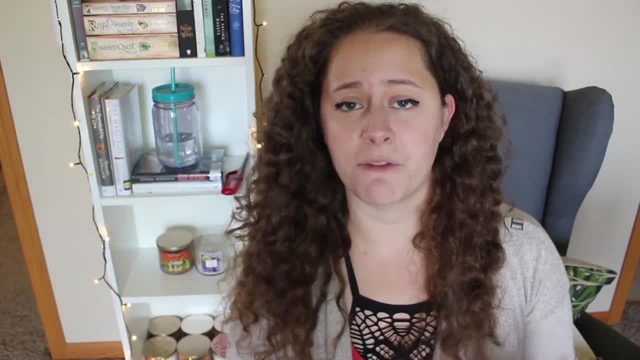 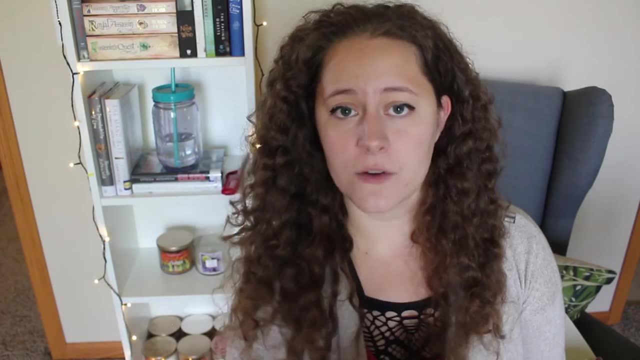 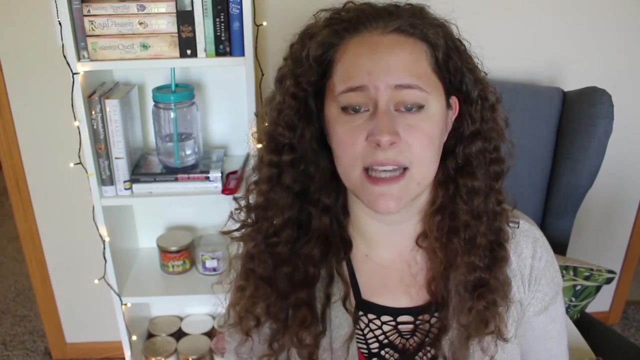 is the technical term for the sloshing back and forth of water. You can recreate this oftentimes in a bathtub and obviously if the seiche goes higher than the banks of the river or lake, it can cause flooding. The next couple are strictly effects of earthquakes, because the damage of human 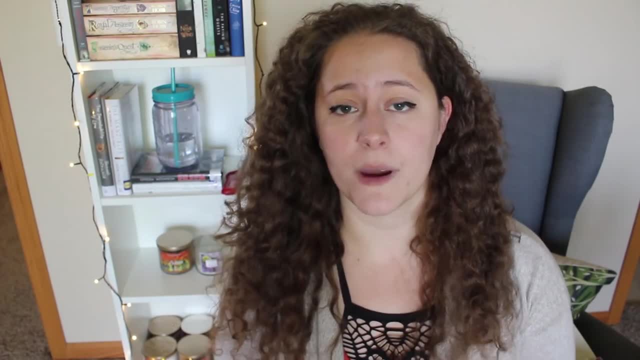 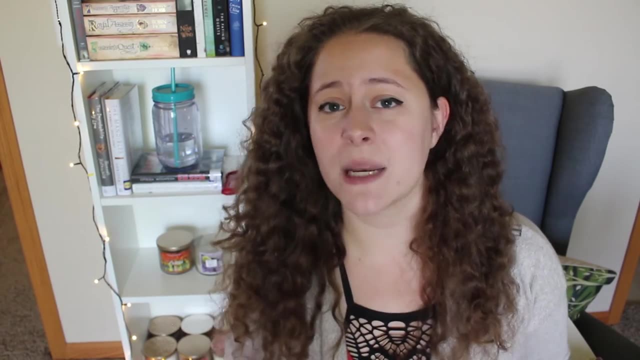 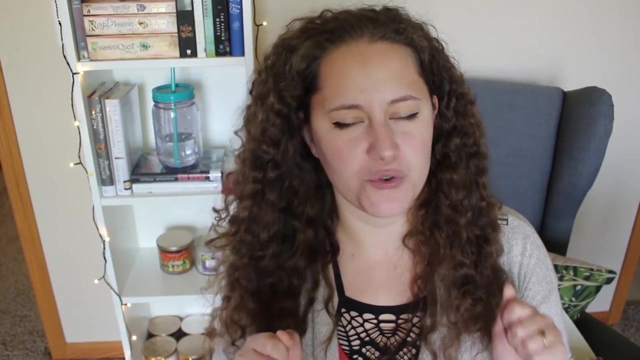 made things. One is fire, and these are caused by breaking electrical and gas lines. In fact, in the case of the San Francisco earthquake of 1906, it is estimated that almost 90% of the damage that was done was actually caused by the fires. If you think of, like maybe one building that really you don't want. affected by earthquakes. high up on that list is gonna be a nuclear power plant, But we probably all remember the Fukushima meltdown. that happened in 2011.. So nuclear power plants are not immune to kind of messing stuff up during an earthquake. This was dangerous not only because the nuclear power core was.